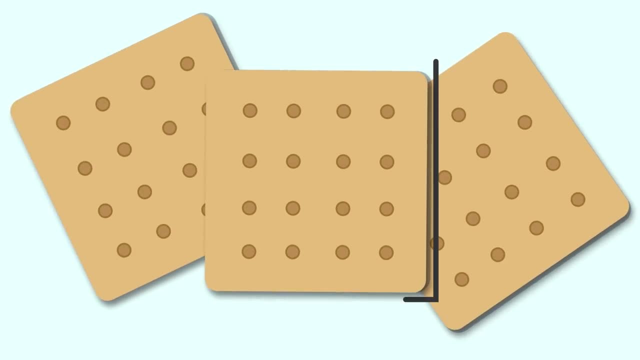 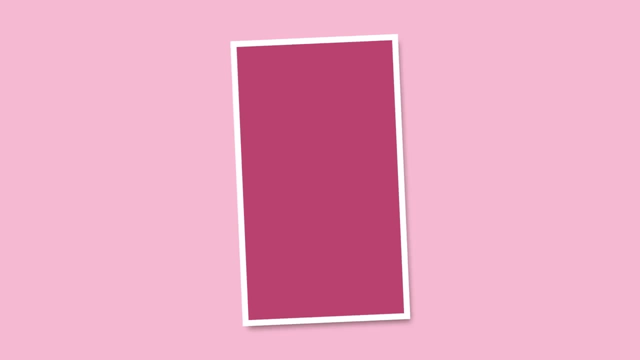 Or like this cookie: No more food talk, I'm feeling really hungry. This is a rectangle. It has four sides, like this square, but they're not identical. Only it's opposite sides are opposite sides, so they are not identical. 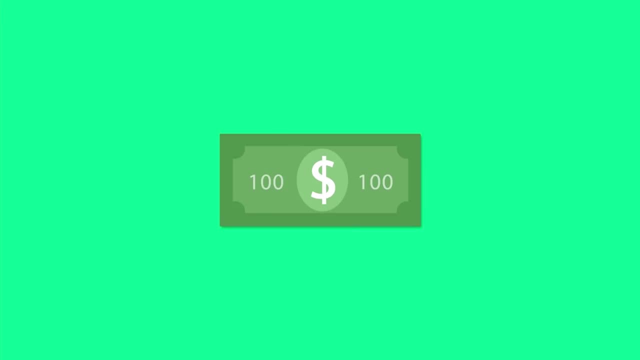 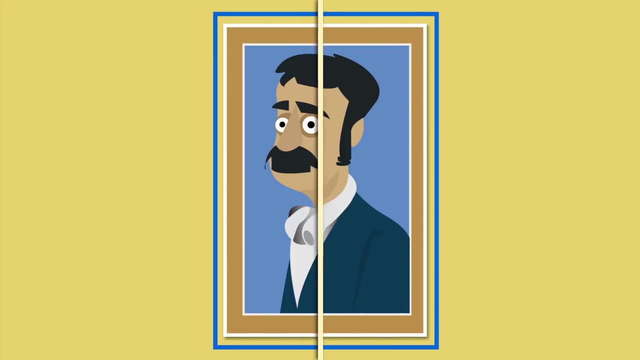 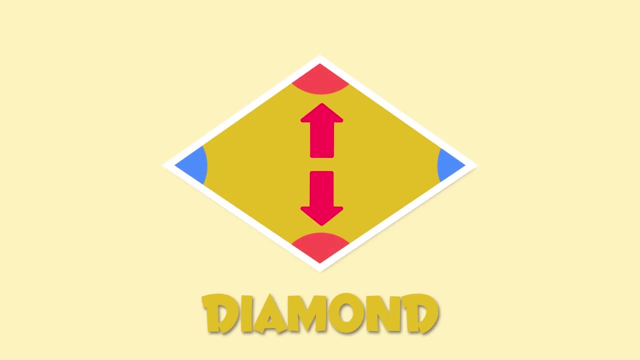 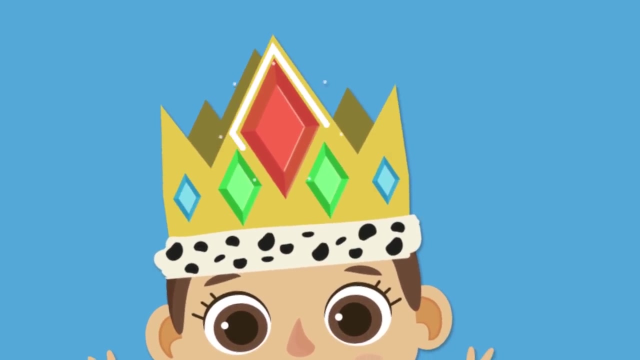 Only it's opposite sides are opposite. sides are equal in length. a rectangle looks like this bill or like this picture frame. this is a diamond shape. its four sides are identical, but its angles are not, meaning this one and this one are equal, and so are these two. a diamond looks like the jewel on this crown or like this kite. 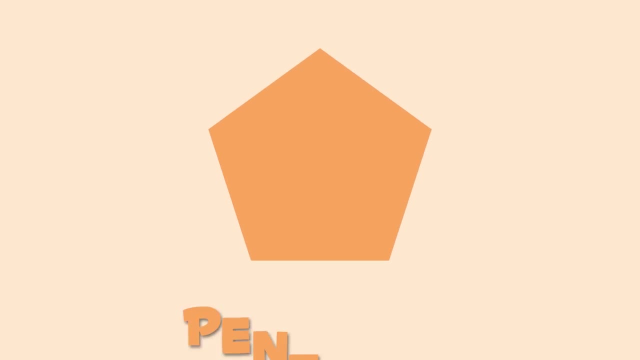 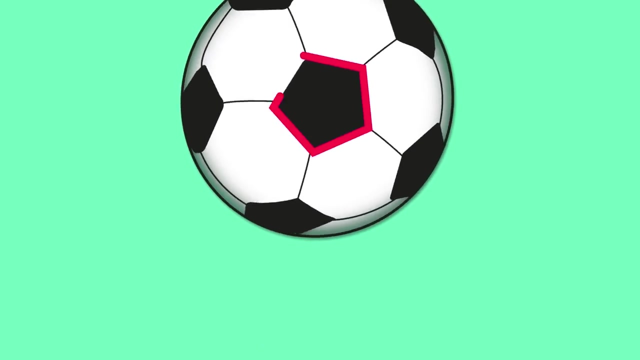 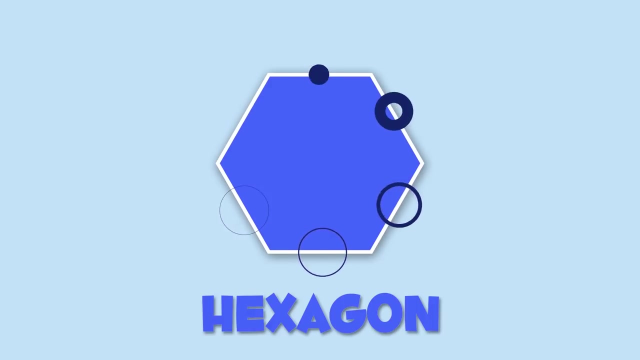 so this one right here is a pentagon. pentagons have five sides: one, two, three, four and five. a pentagon looks like this birdhouse or like these football stitches. finally, i'll show you the hexagon. hexagons have six sides. a hexagon is like this stop sign. 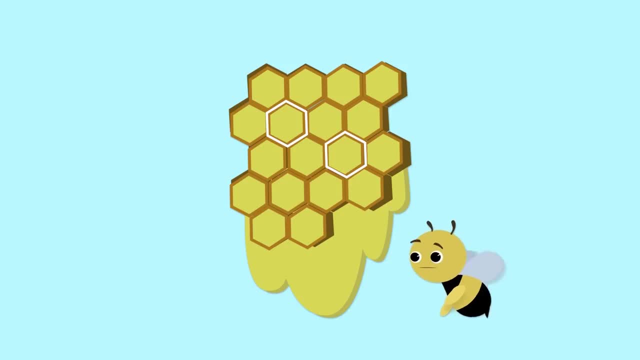 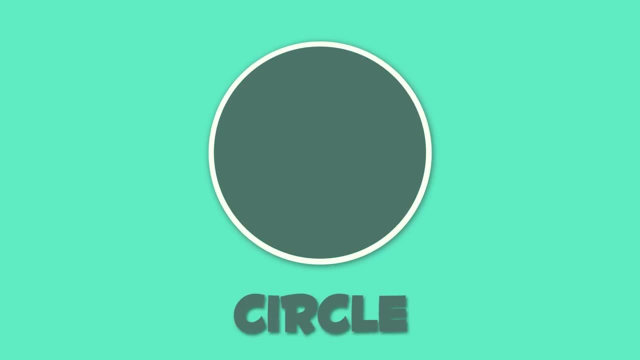 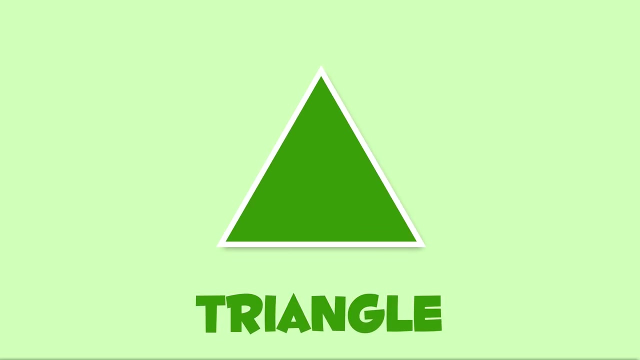 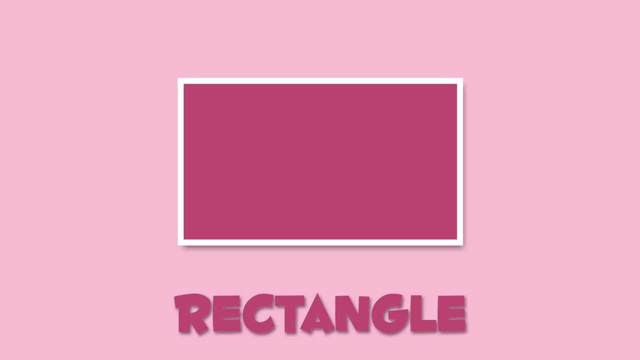 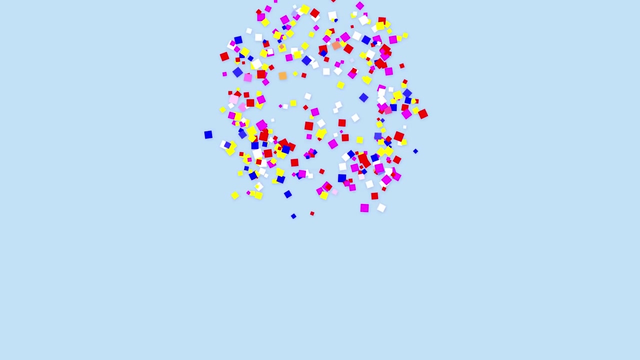 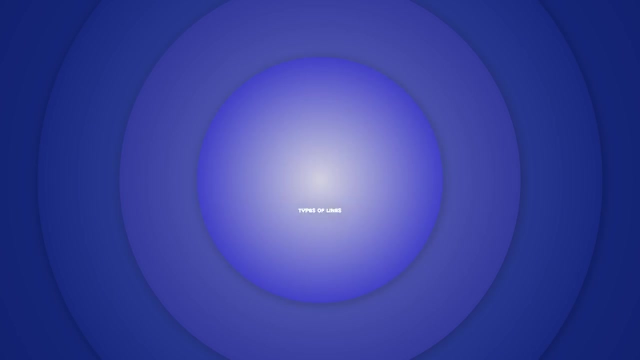 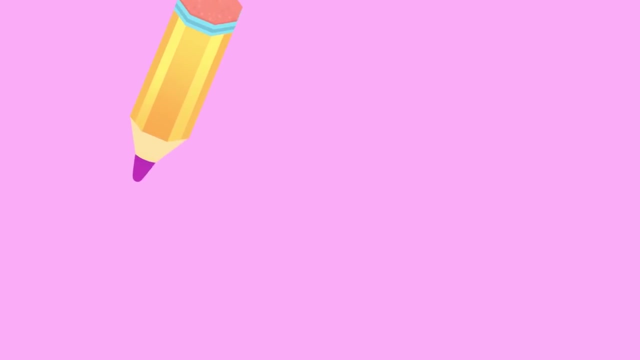 or like this: beehive, we better go now. bees are getting angry. recap: circle, oval triangle, square rectangle, diamonds, pentagon, octave 2: points 1, 2, 4, 5, 6, 7, 8, 11, 12, 7, 14, 15. 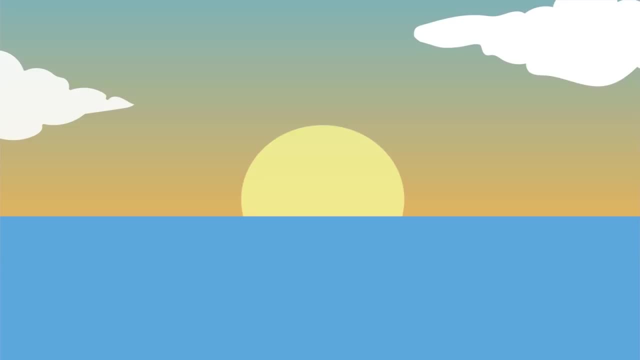 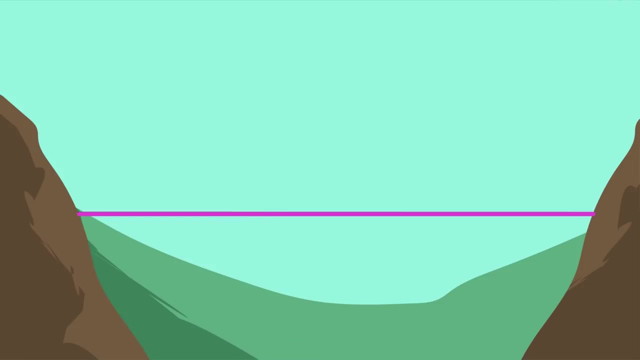 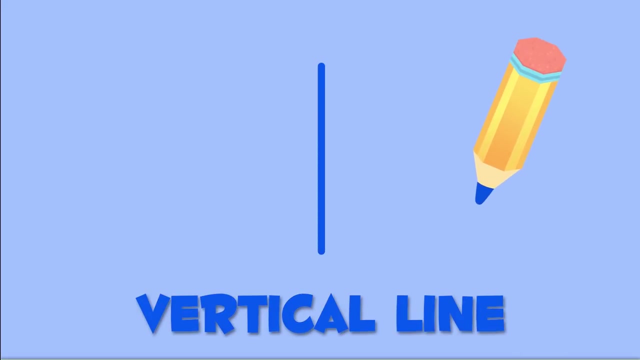 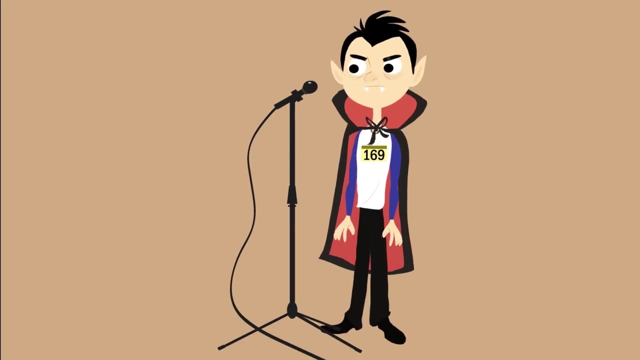 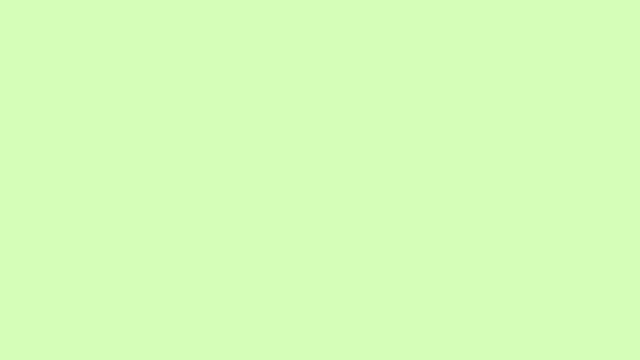 14 Horizontal lines. look like the horizon, Or like the tightrope of an acrobat: Whoops cheerio. Now, this is a vertical line. Vertical lines look like the trunk of this palm tree, Or like this microphone. stand Bass, keep practicing. 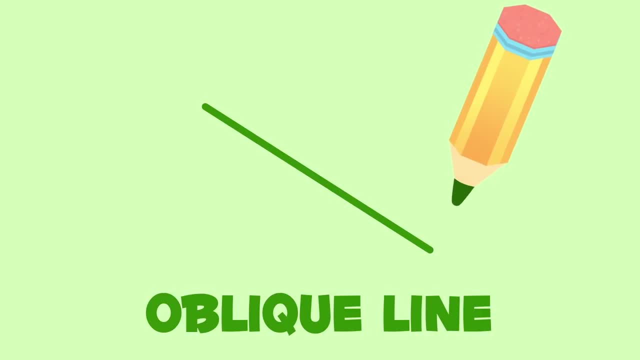 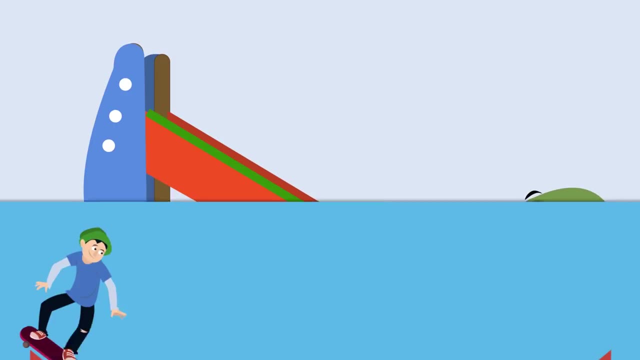 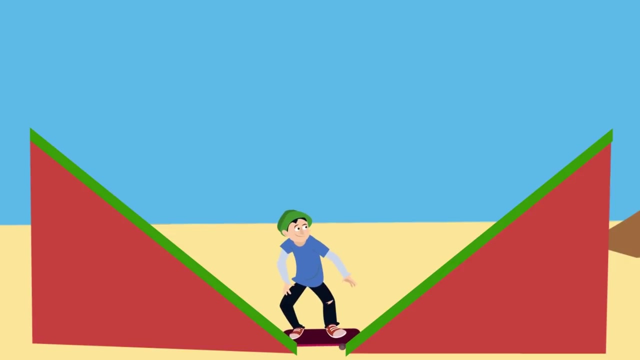 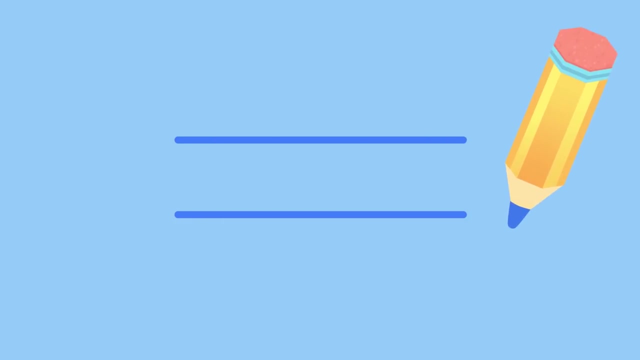 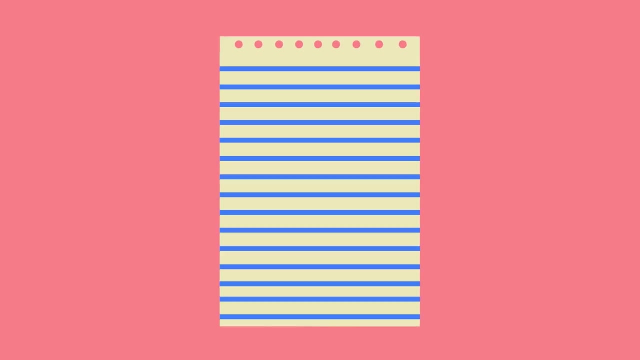 This is an oblique line, Oblique lines. look like this slide Or like this skateboarding ramp: Wow, so fast. Now here's two lines, One next to the other. They're called parallel lines because they never touch The lines in this notebook or the steps of this ladder are parallel. 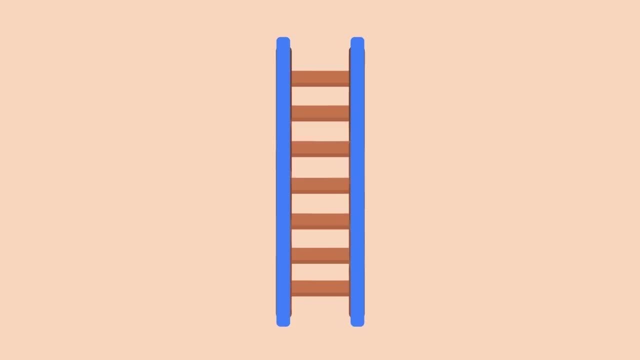 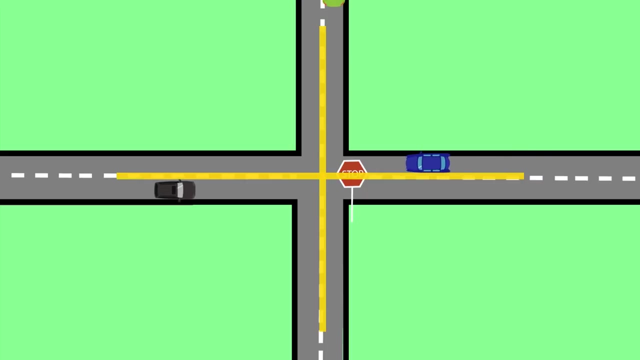 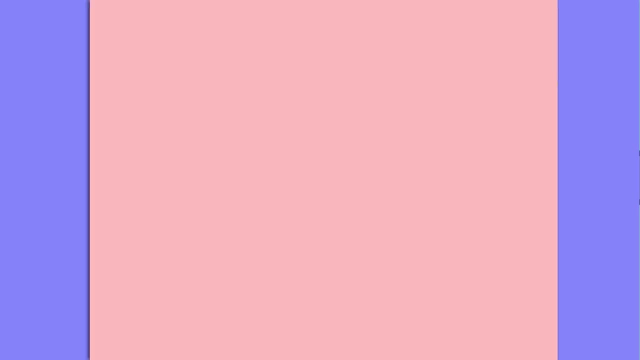 We can turn a parallel line to make it vertical. When parallel lines crisscross, they change to perpendicular lines. Perpendicular lines look like this crossroads Or the frame of this window. What a lovely day. Straight lines can also be polygonal. 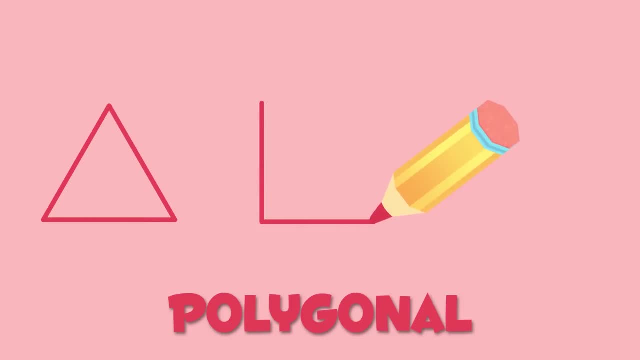 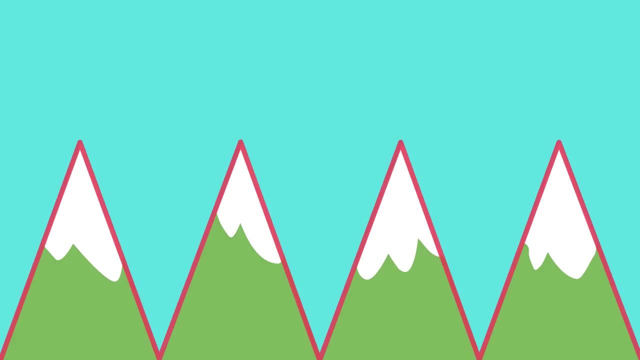 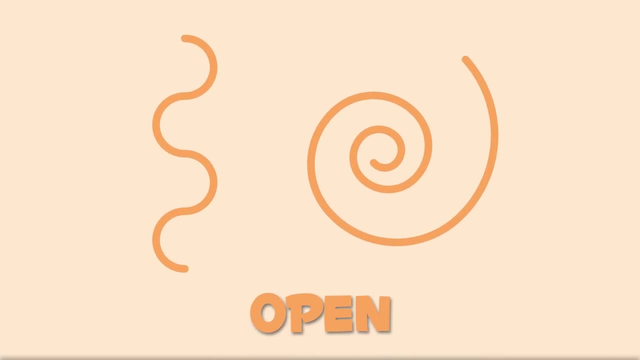 Or closed, like this triangle, The square Or the pentagon. Straight lines can be open too, Like these ones, for example. They look like mountains. Let's have a look at curved lines. Curved lines can be open Or closed. 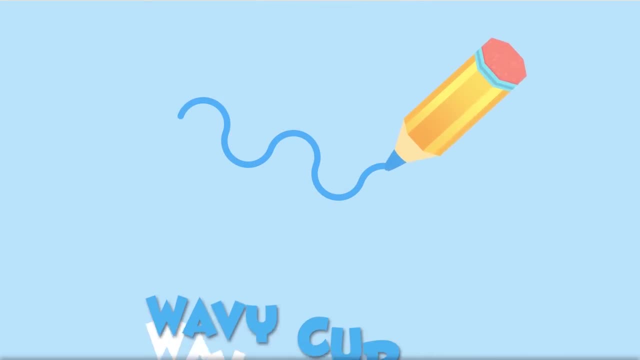 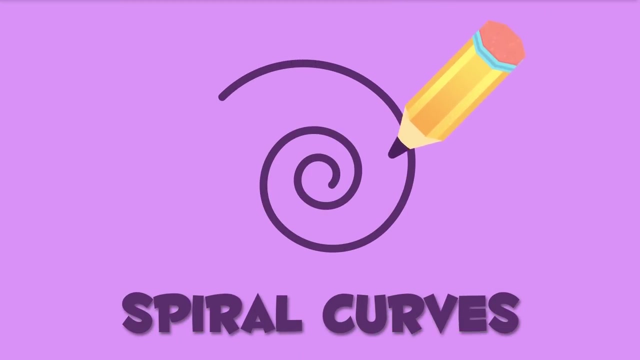 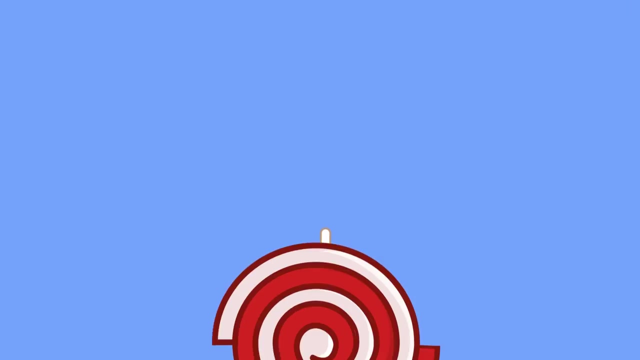 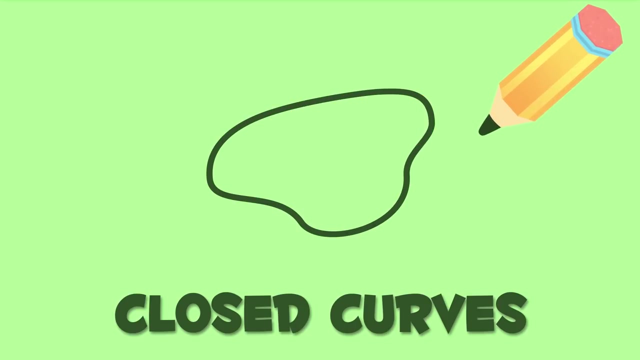 Wavy curves are in the same group as curved lines, Like this curvy path Or this worm. Spiral curves are in the same group as open curves, Like this snail Or this lollipop- So yummy, So yummy. Close curves are like this pond. 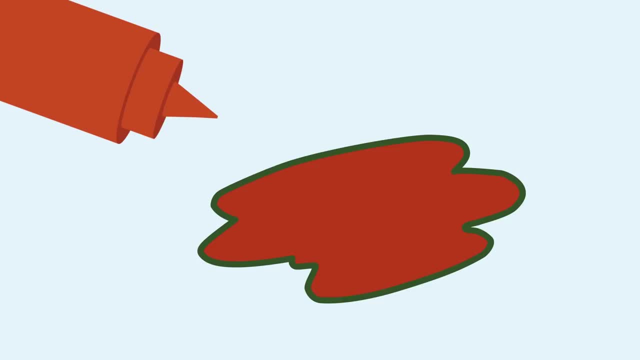 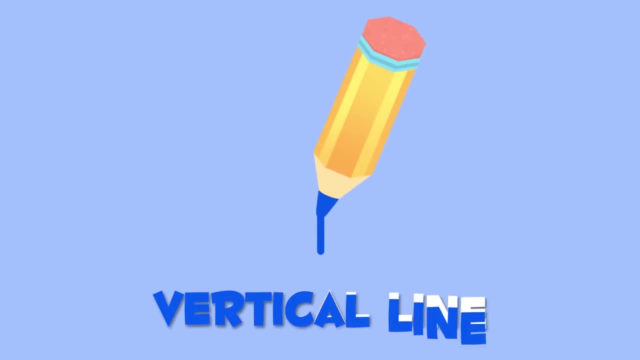 Or this ketchup stain. Awesome. Let's recap: Horizontal line, Vertical line, Oblique line, Close curves are like this pond Or this ketchup stain Or this nut. Parallel lines, Perpendicular lines, Closed polygonal lines. 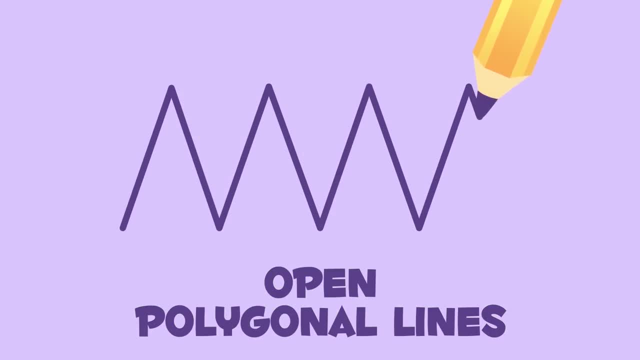 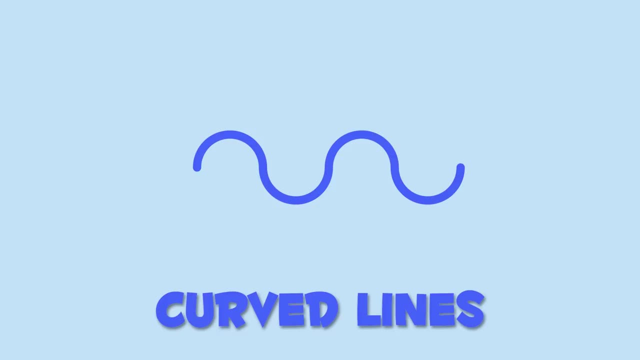 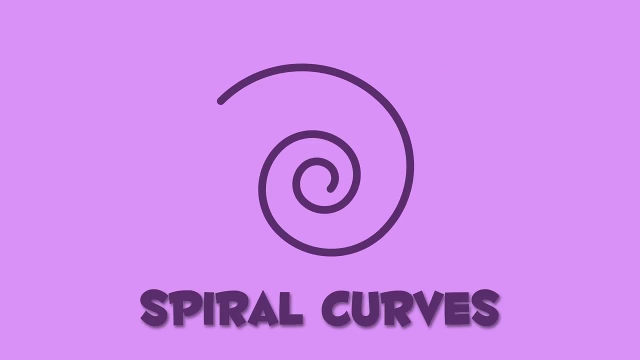 Opened polygonal lines, Curved lines, Up and down, From side to side, To the right, to the left, To the left, to the right, To the left, to the right, To the right, Spiral curves, Closed curves. You learned everything about all types of lines. 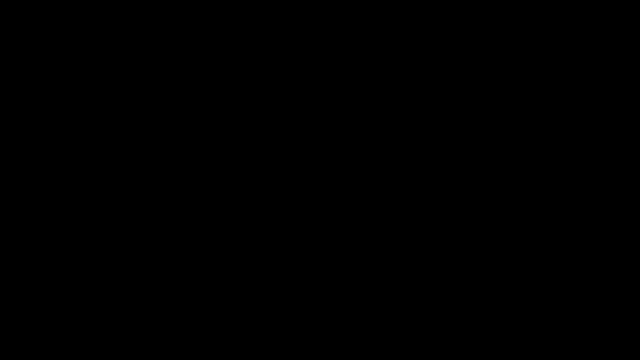 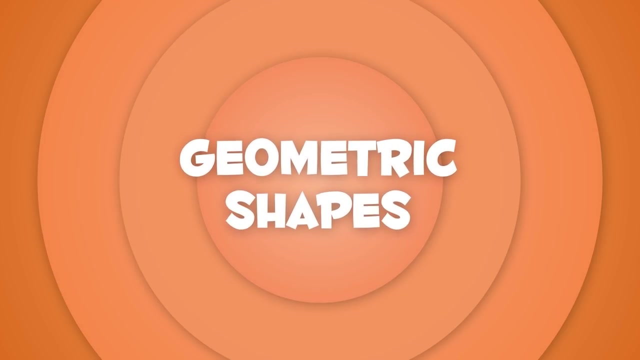 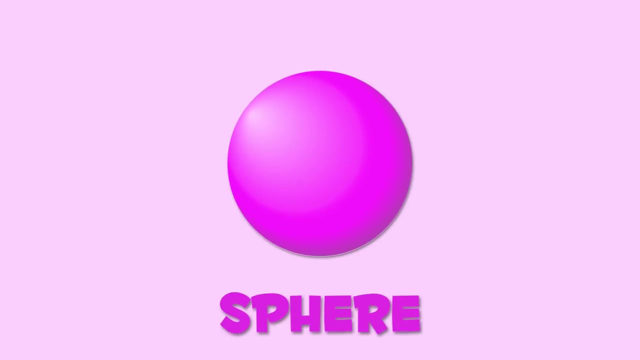 Well done. Today we're going to learn about geometric shapes. Do you know how many types are there? Here they come. Take a guess. What is this? Yes, it's a sphere- Spheres. look like this tennis ball Or like this bowling ball. 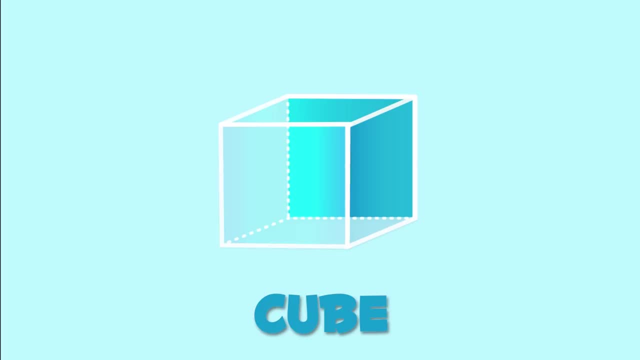 And this is a cube. Cubes have four identical square sides. Dice are cubes, Dice are cubes. And this box is also a cube. This shape is a cylinder. Cylinders have two identical flat circular bases. A cylinder is like this: can. 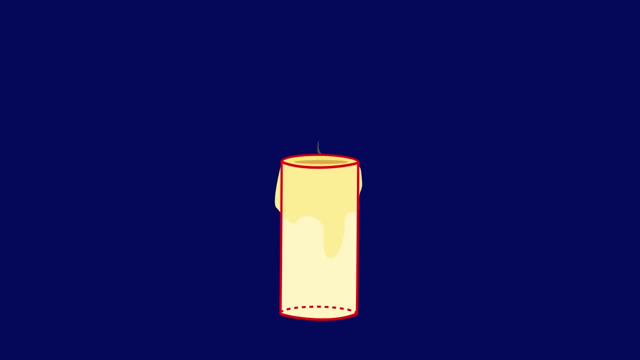 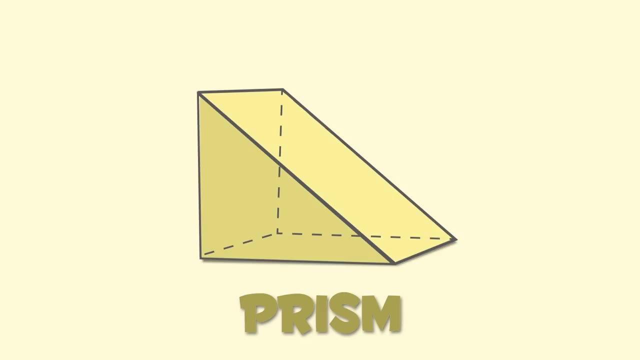 Or like this candle. This is a prism. Both faces of the prism are identical. There are many types of prisms. This milk carton is a prism. As you can see, both of its faces are identical squares, But in this prism its bases are triangles. 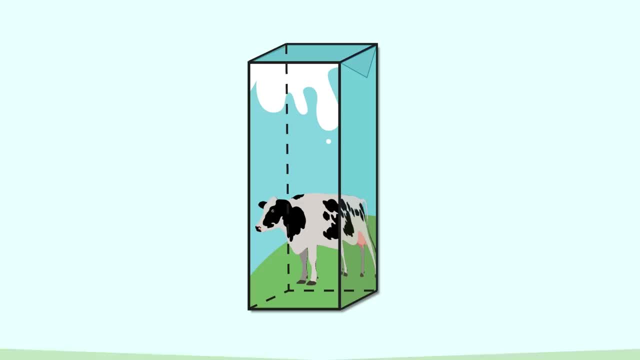 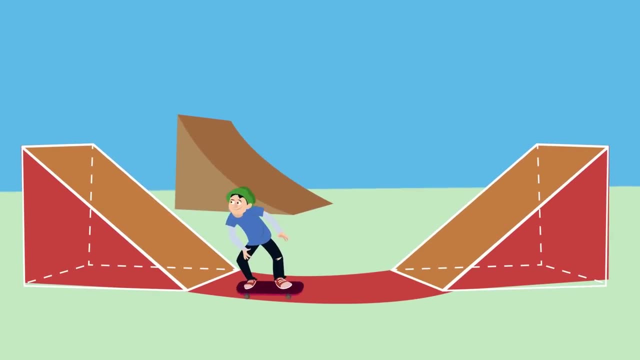 It looks like a skating rink. Wow, so fast. This one is super easy. I'm sure you've seen it before: It's a pyramid, Its base is a polygon And its sides are triangles. All sides meet at a central point. 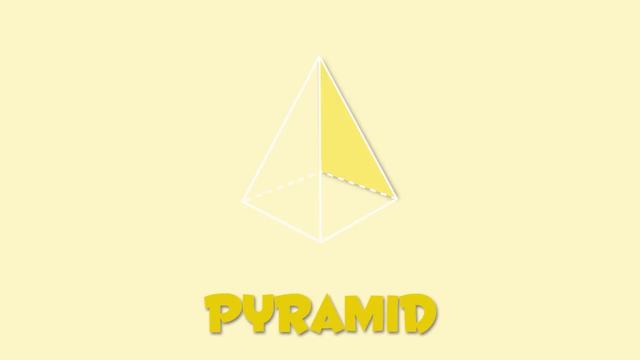 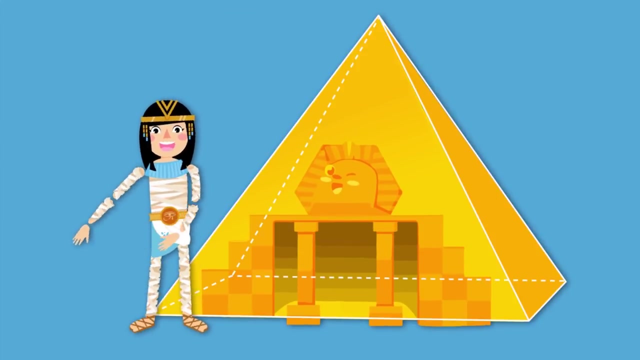 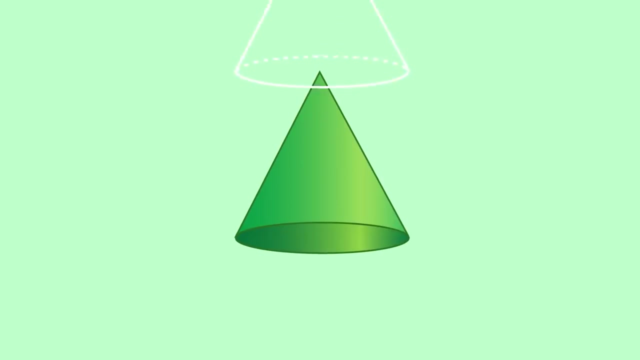 It's a pyramid. It's a pyramid. It's a pyramid And its sides meet at a central point, The apex, Just like the pyramids in ancient Egypt, Or like this Indian-style tipi. Finally, I'll show you a cone.